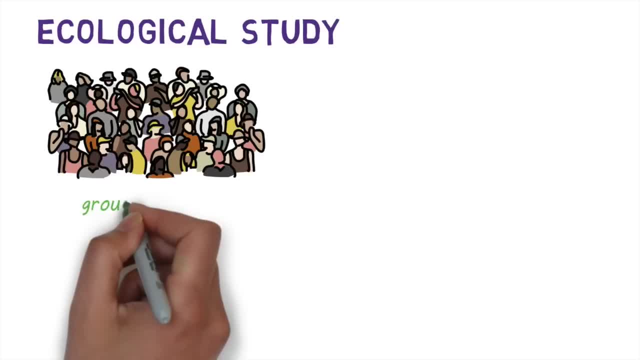 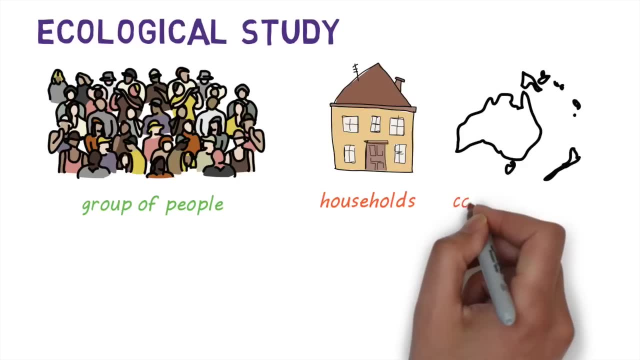 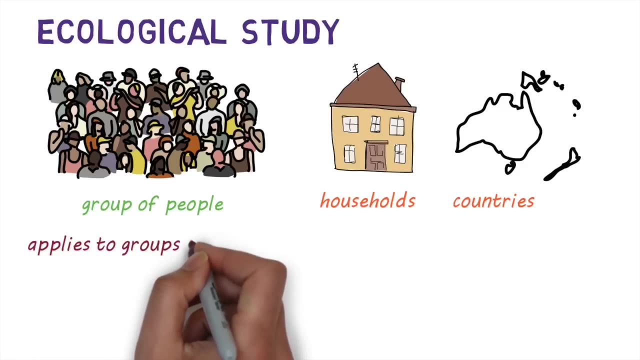 where measurements like disease rates and information about exposures are made on a group of people. The groups can be as small as people in a house or as large as people in an entire country. remember that results and conclusions from ecological studies apply to a group and not to individuals. Ecological studies are useful for comparing the 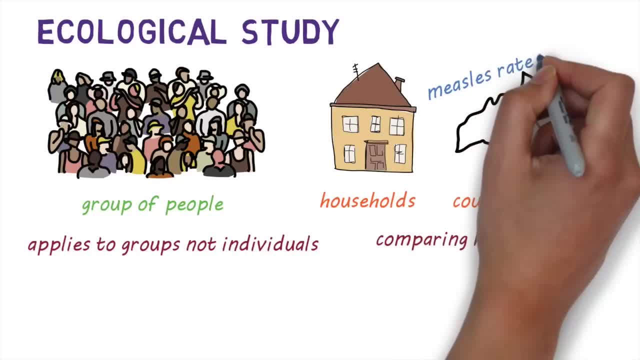 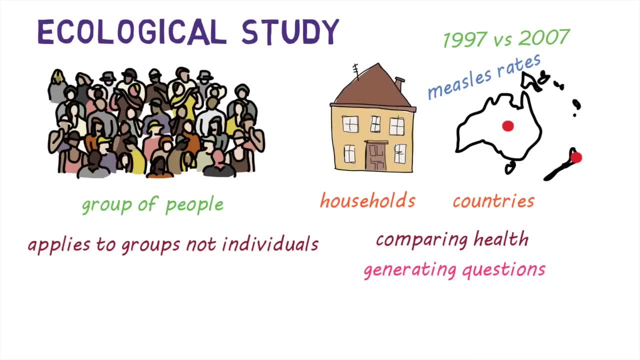 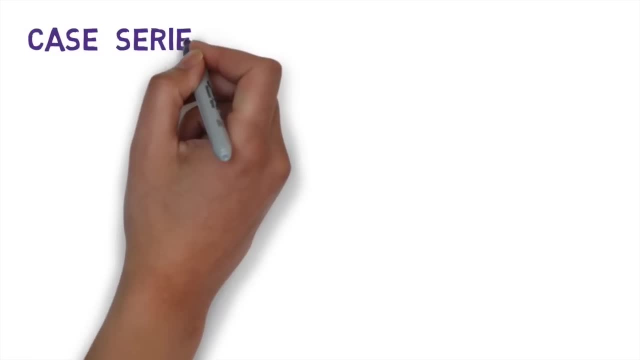 health of populations in different places, such as measles rates in Australia and New Zealand, or at different times. They're also useful for generating questions and highlighting issues that can lend themselves to future investigations or studies. A case series describes the characteristics of a group of people who have the same disease or the same exposure. The aim of 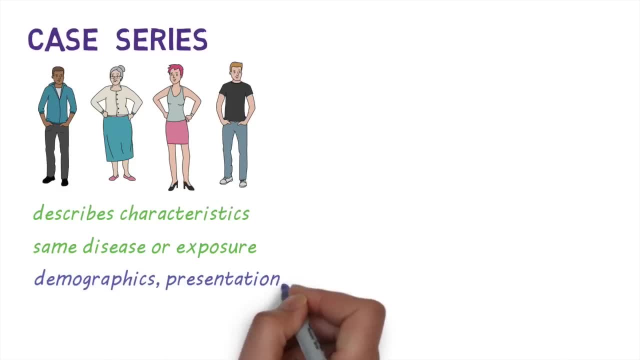 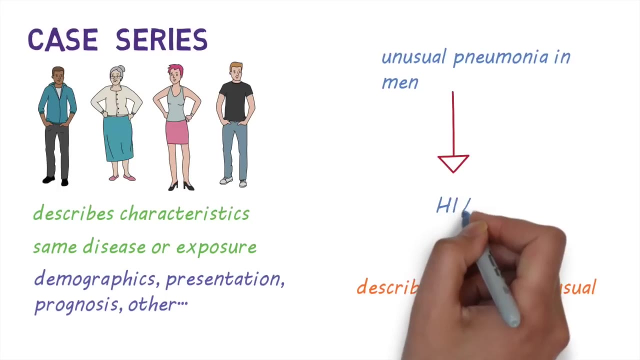 this is to understand the demographics, clinical presentation, prognosis or other characteristics of people who have a particular disease or describe something unusual. For example, in the early 1980s, the occurrence of an unusual pneumonia in men led to the recognition and identification of HIV, A cross-sectional 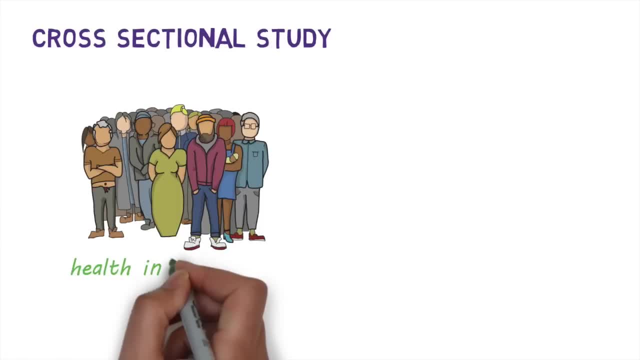 study takes a selected population and measures health information at a given point in time, giving a snapshot of their health. It usually involves asking participants a series of questions using a questionnaire. Health surveys that collect health information about people in a population is an example of a. 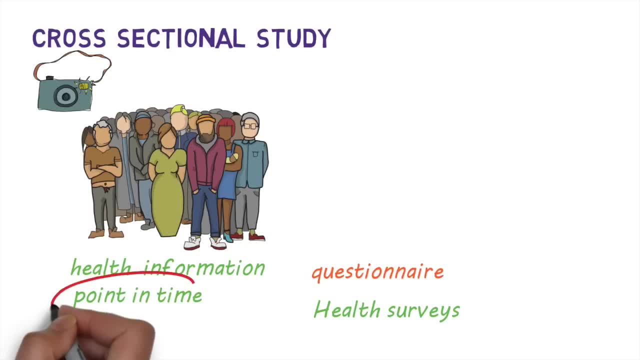 cross-sectional study. Because these studies commonly measure how many people have a disease at a particular point of time. they're also called prevalence studies. It's important to make sure that the selected population is representative of the total population. Cross-sectional studies are relatively inexpensive and easy to conduct compared to other studies. They 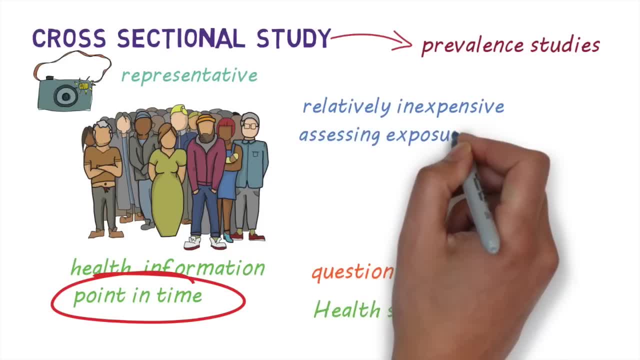 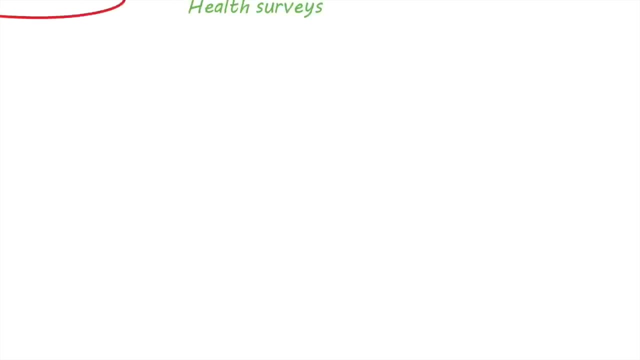 can provide information on multiple exposures and outcomes and are a good way of assessing the health needs of a population. However, because the information is collected at a single point in time, it cannot be used to determine whether a particular exposure caused the disease or not. A case control. 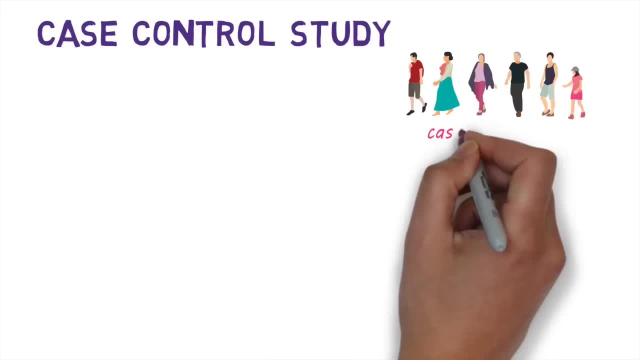 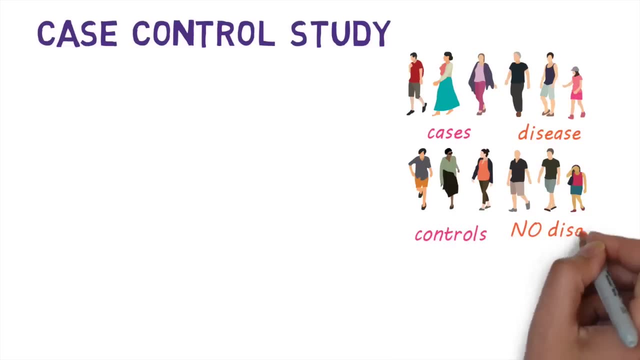 study starts off with cases. These are people with a disease. It uses a comparison group called case control case, but do not have the disease. Both groups are asked about their previous exposures to different risk factors For each of the list. fact here's: 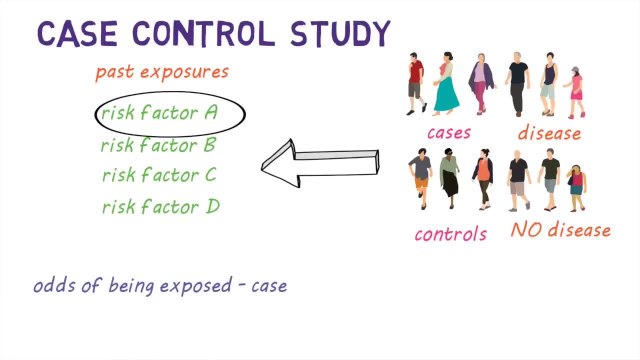 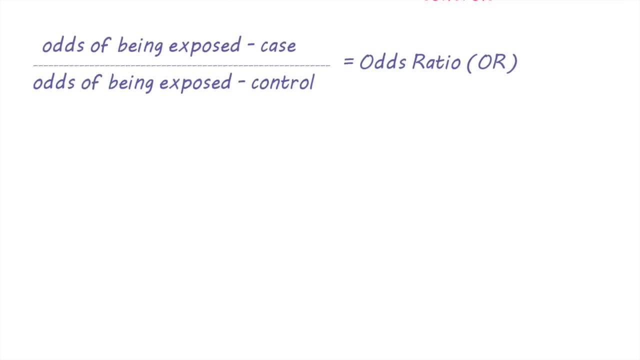 the odds of being exposed if they were a case is compared to the odds of being exposed if they were a control. This is called an odds ratio. An odds ratio of more than one means that people with the disease are more likely to have been exposed to that risk factor- the people without the disease. This suggests that 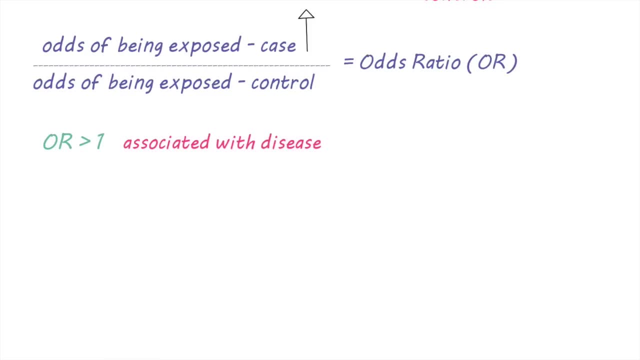 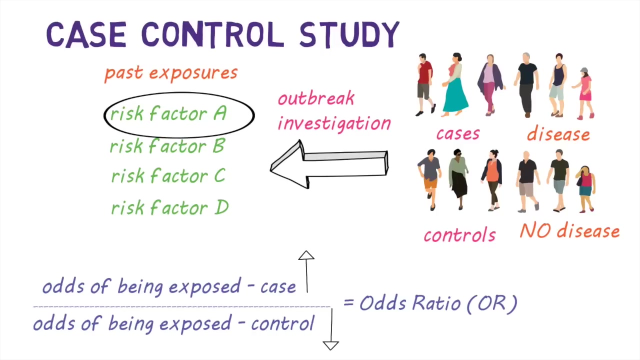 it could be a possible cause of the disease. An odds ratio of less than one suggests that it's a protective factor and one suggests no association. Case control studies are commonly used in foodborne outbreak investigations. For example, we can compare the odds of eating. 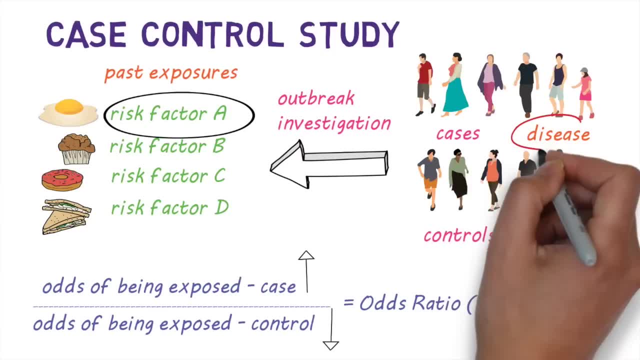 different kinds of food, between people who fell ill after consuming a meal and those who didn't. If the odds ratio is greater than one for a particular type of food, then it's possibly the cause of the illness. A major advantage of a case control study is that they're often quick and cheap to do. 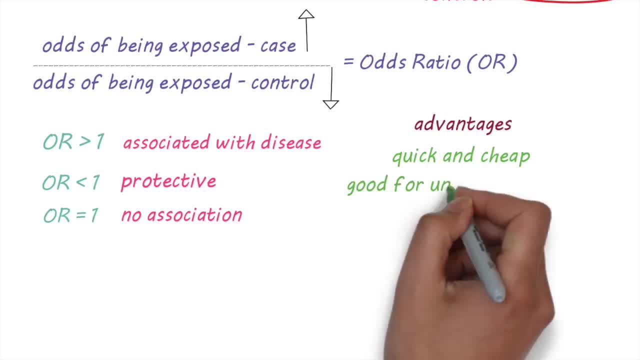 Also, because they start off with cases, it can be used to study uncommon diseases. However, because these studies involve small numbers, they're not good to study rare exposures. One of the challenges in a case control study is to find suitably matched controls Also. 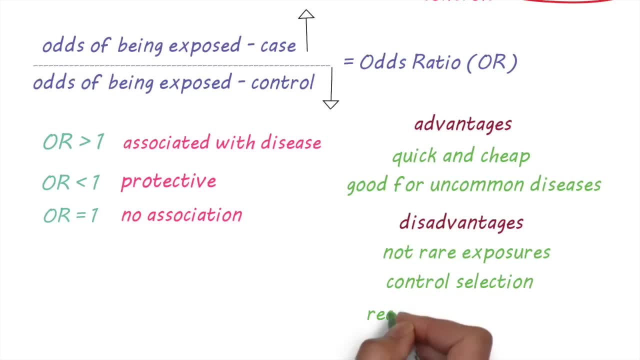 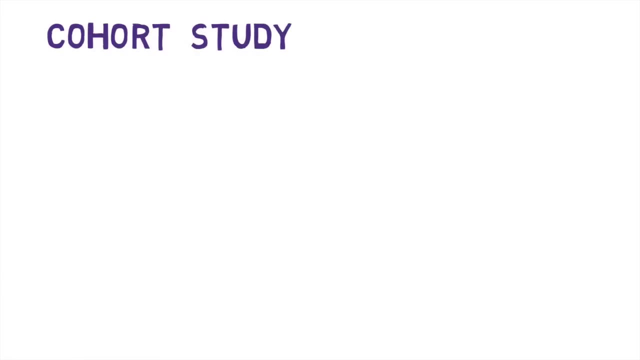 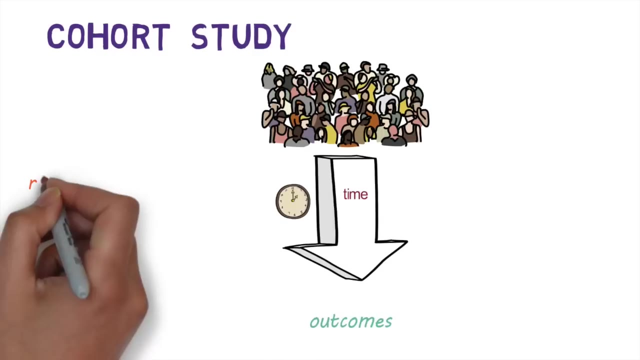 because studies ask about exposures in the past, people might not be able to recall their exposures accurately. Let's have a look at cohort studies now. In a cohort study, a group of people is followed over a period of time to see what happens to them, and information about risk factors is collected. 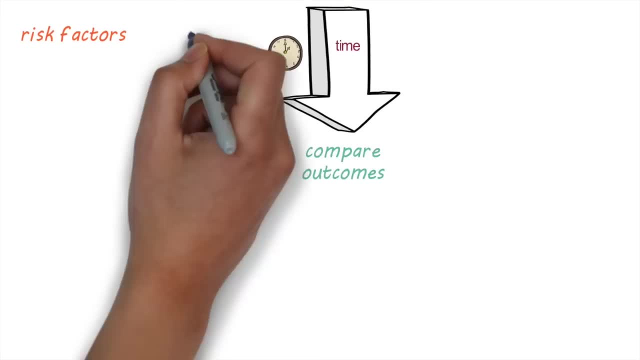 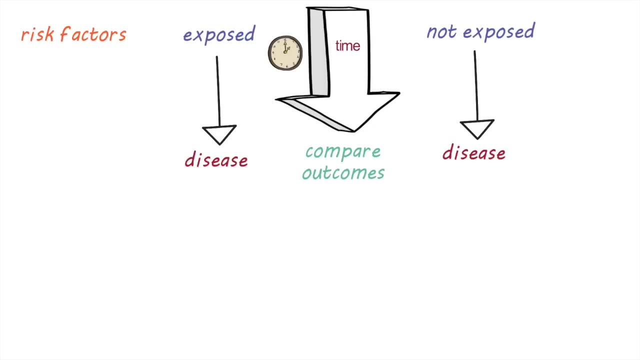 We can then compare the occurrence of an outcome like disease in those who are exposed to a particular risk factor to those who were not exposed to that risk factor. The main measurement used in cohort studies is called the relative risk. A relative risk is the ratio between the risk of disease and the exposure to manifest factors. 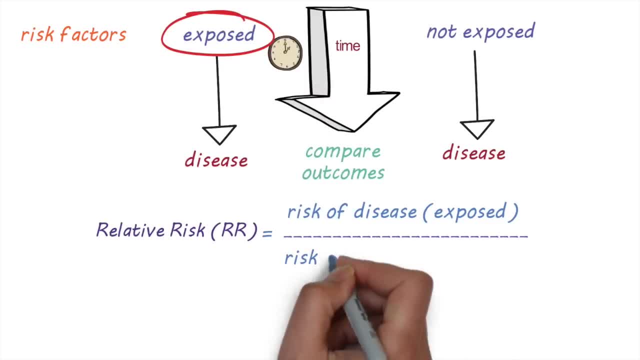 group compared to the risk of disease in the unexposed group. a relative risk of greater than one means that the exposure is associated with an increased risk of the disease. if it is one, it indicates that the risk is the same, and if it's less than one, it indicates that the risk is lower. a well-known cohort study is: 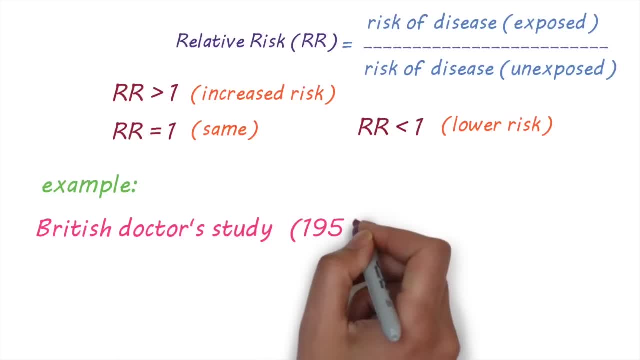 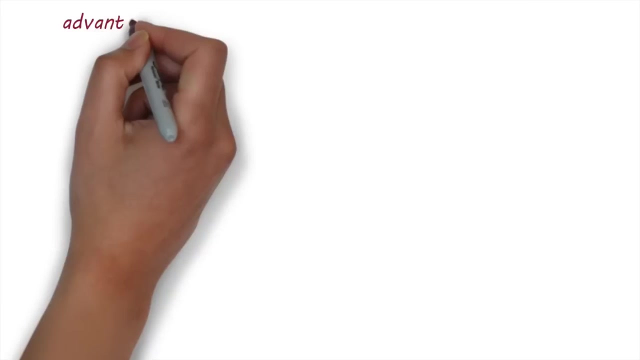 the British doctor study done in the 1950s, where a group of doctors were followed up for many years. this study provided valuable scientific evidence of the harmful effects of smoking, especially the link between smoking and lung cancer. one of the main advantages of cohort studies is that the time 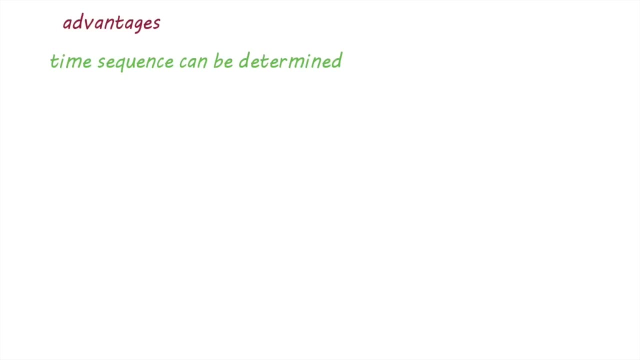 sequence of events can be determined. this is useful when trying to determine what caused a disease. another advantage is that information about several different outcomes and risk factors can be collected at the same time. this allows for sub analysis to be conducted on the data you. a disadvantage of cohort studies is the high cost, as they can involve a large 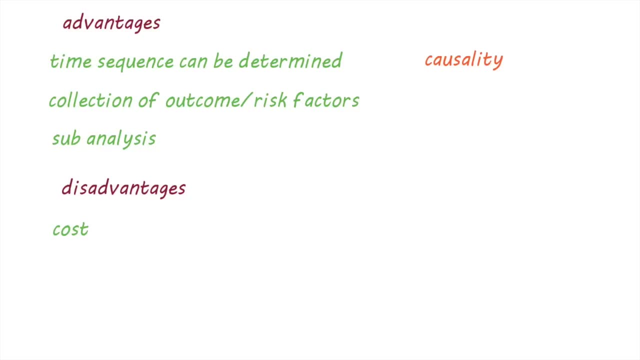 number of people being followed over a long period of time, they're generally not suitable to study rare diseases. a challenge in cohort studies, especially ones that are conducted over a long period of time, is ensuring that people who started the study stay until the end of the study, if many people drop out it. 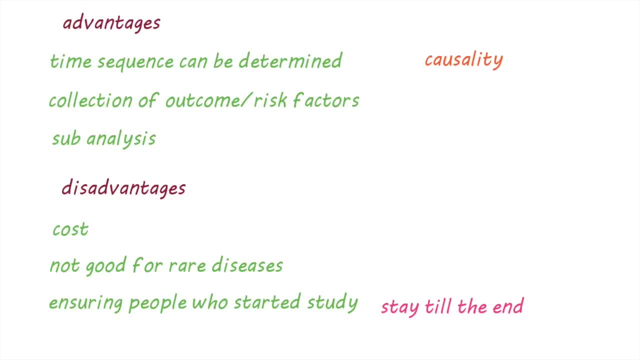 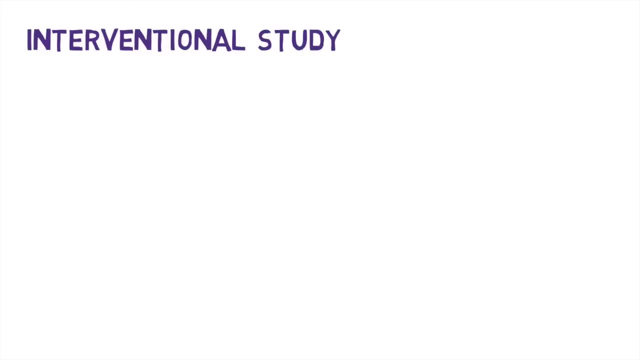 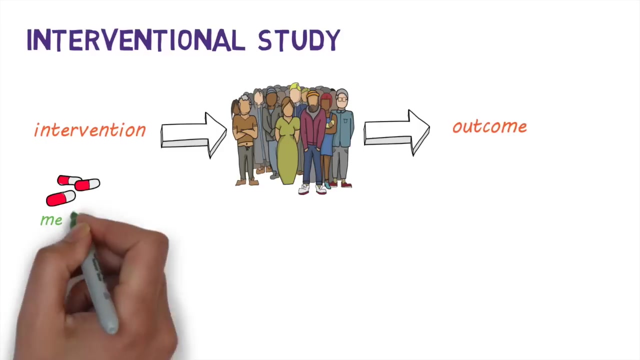 will affect the results of the study. now let's look at another type of study: an interventional study. in an interventional study, an intervention is done on a group of people and the outcome studied. examples of interventions can be giving a medicine, a vaccine or health advice. the outcome can be things like a change in disease. 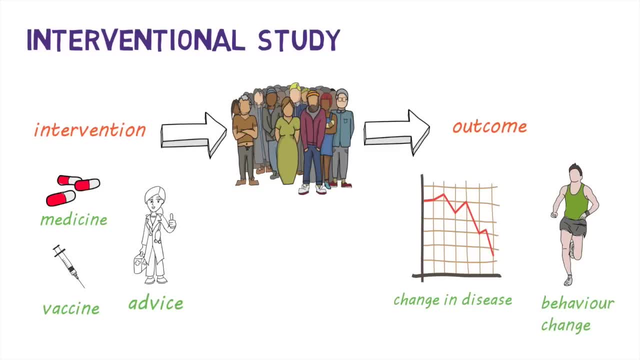 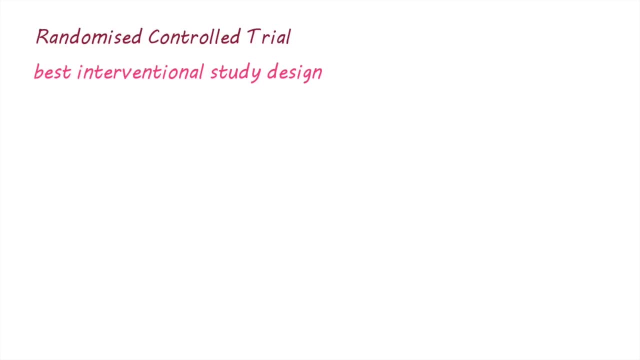 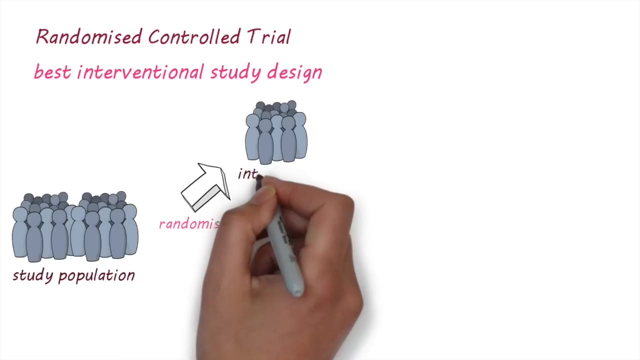 status or change in behavior. a randomized, controlled study is the best study design for an interventional study. say, we want to study the effects of a new drug off with a study population. People are then randomly allocated to be in the intervention group, where they receive the drug, or in the control group, where they don't receive. 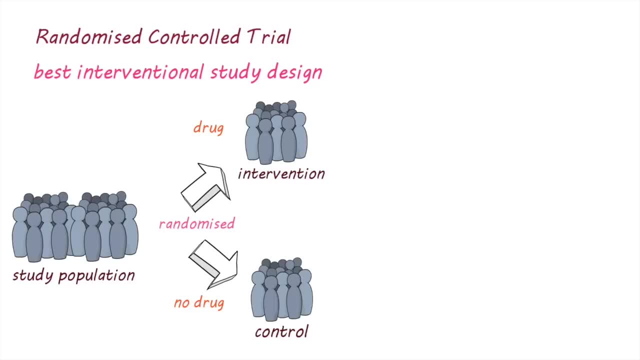 the drug. Then, after a suitable time period, the outcomes in the two groups are assessed and compared to see what effect the drug had. Outcomes can be things like a change in disease symptoms or death rates. Ideally, neither the participants nor the 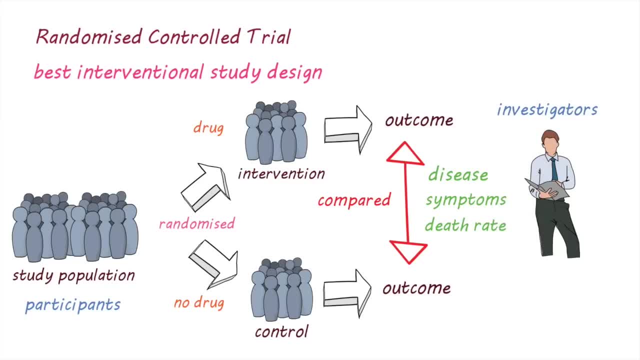 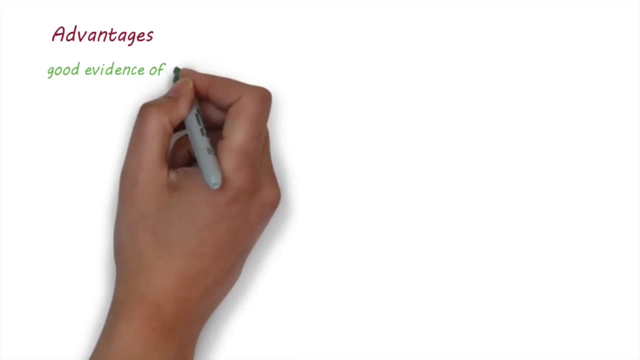 investigators should know which group received the intervention. This is called double-blinding and ensures that neither of them can influence the outcome of the study. The main advantage of a randomized control study is that it can provide good evidence that the intervention led to an outcome. Randomization ensures that both groups have an equal chance.